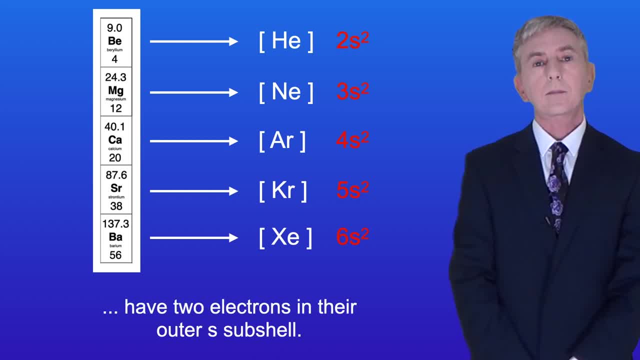 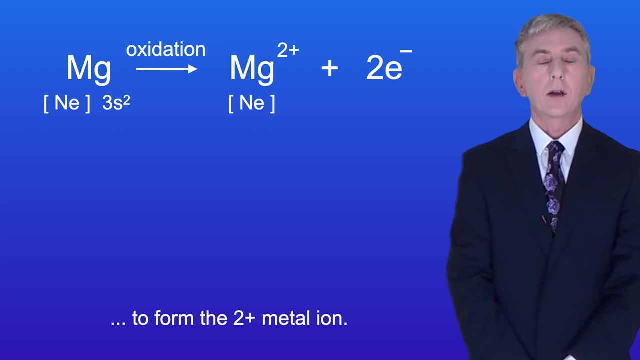 2 elements have two electrons in the outer S subshell. When Group 2 elements react, they lose these outer two electrons to form the two positive metal ion. and I'm showing that here for magnesium. Because it's losing electrons, the Group 2 metal is being oxidized. These two electrons 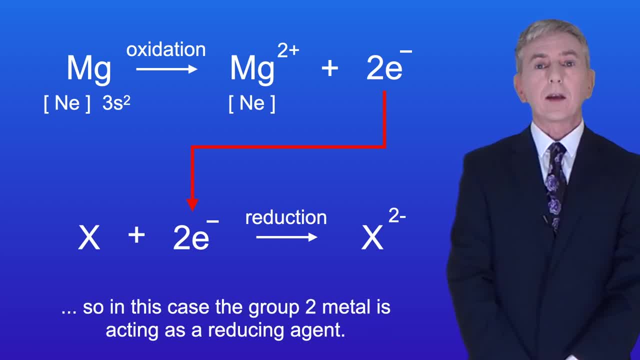 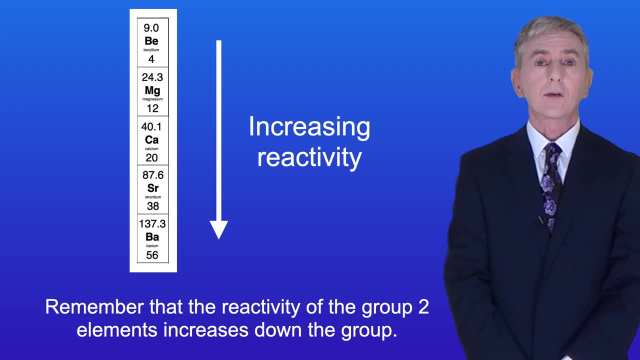 can then be used to reduce another chemical. So in this case, the Group 2 metal is acting as a reducing agent. Remember that the reactivity of the Group 2 elements increases down the group. This is because, moving down the group, the first and second ionization energies decrease and 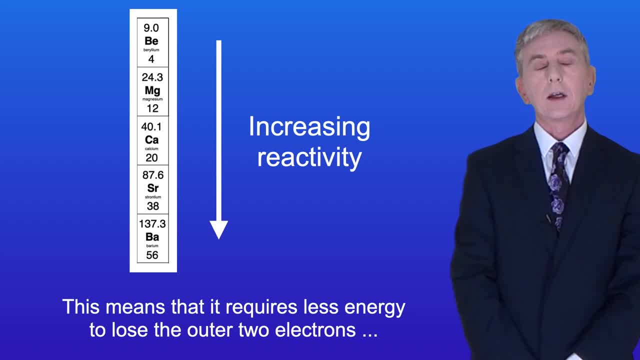 this means that it requires less energy to lose the outer two electrons as we go down the group. I should point out that for the A-level specs we only need to consider magnesium to barium. We're going to start by looking at the reaction with oxygen. I'm showing you here the reaction. 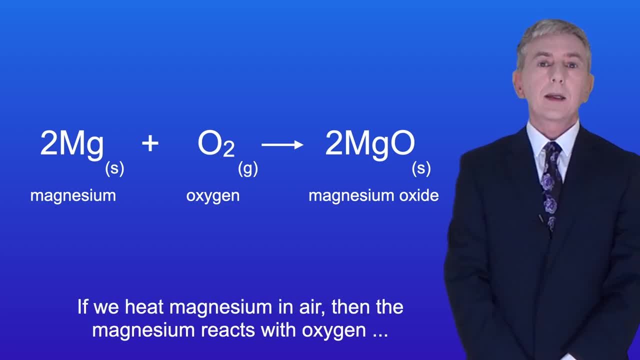 between magnesium and oxygen. If we heat magnesium in air, then the magnesium reacts with oxygen, producing a bright white light. Now this is an example of a redox reaction, and we can show that by using oxidation numbers. I should just remind you that when we write oxidation numbers, we always write them in. 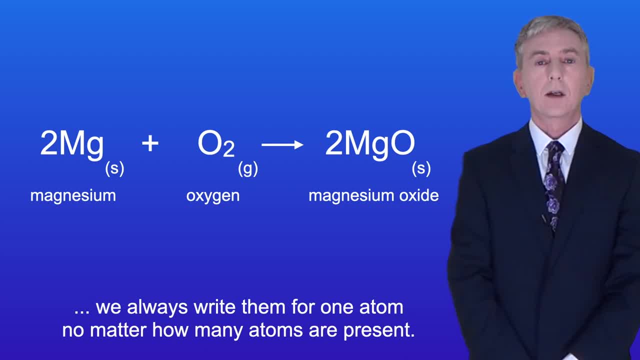 for one atom, no matter how many atoms are present, and remember that elements have an oxidation number of zero. Before the reaction, both the magnesium and the oxidant have an oxidation number of zero as their elements. During the reaction, each magnesium atom is oxidized, losing two electrons. 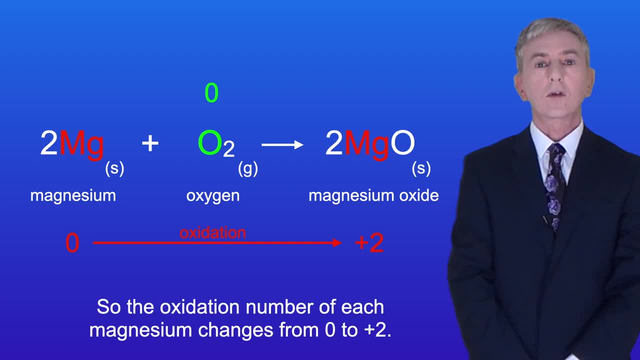 so the oxidation number of each magnesium changes from zero to two. Each oxygen atom is reduced, gaining two electrons. so the oxidation number changes from zero to plus two of each oxygen changes from zero to minus two. Now, a key idea you need to understand is that 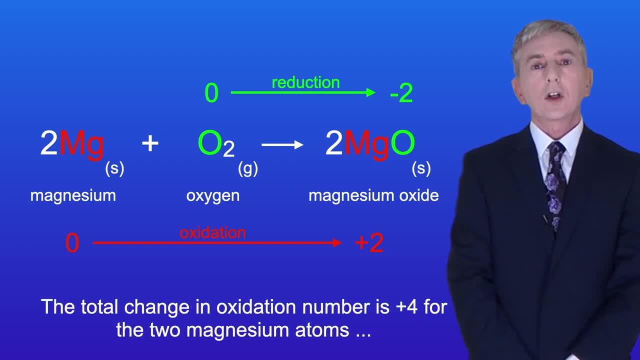 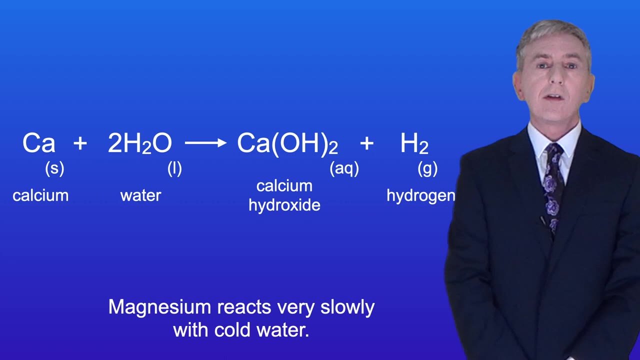 the changes in oxidation numbers must balance. The total change in oxidation number is plus four for the two magnesium atoms and minus four for the two oxygen atoms. Okay, now we can also react group two elements with water. Magnesium reacts very slowly with cold water, but as we move down group two, the elements react more rapidly. I'm showing you.